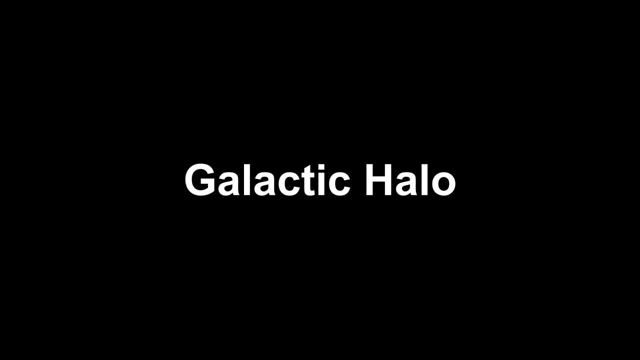 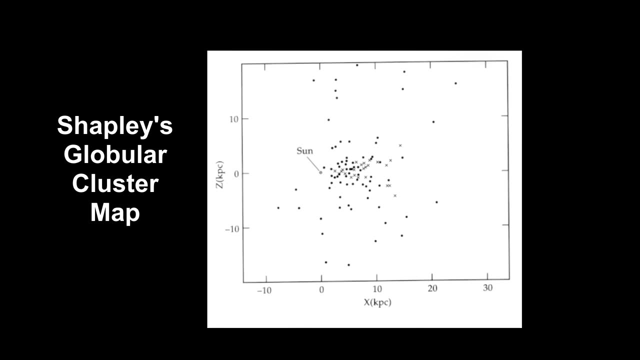 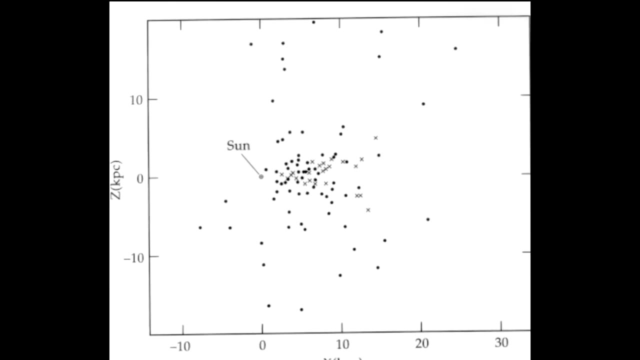 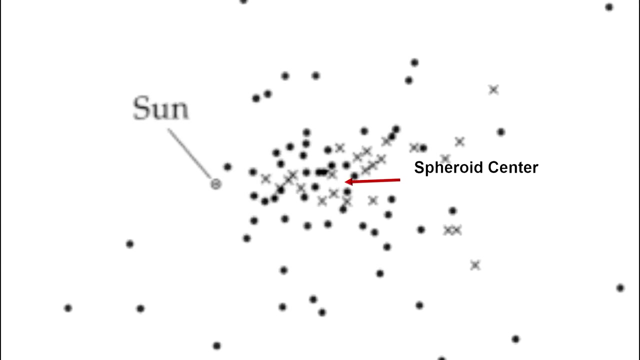 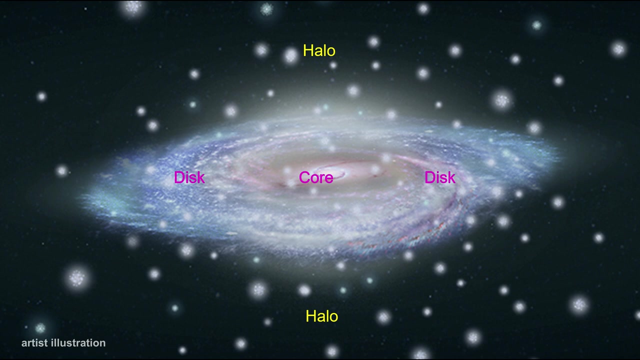 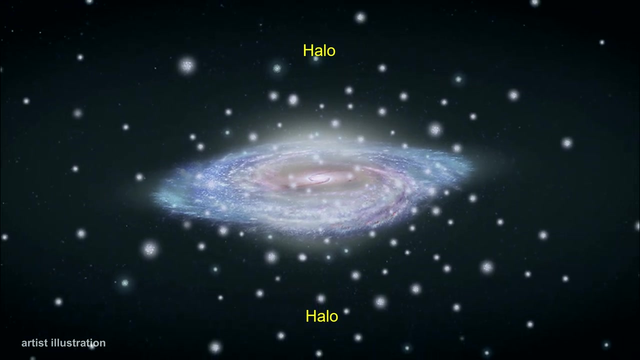 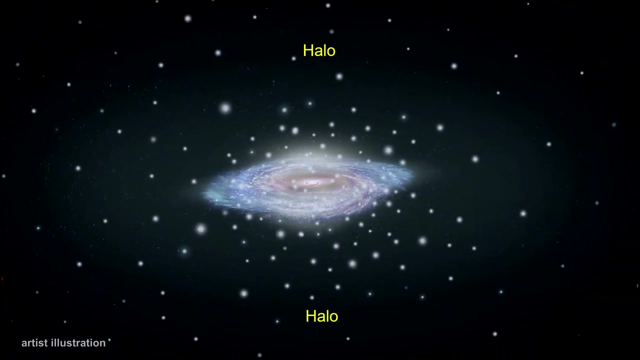 Transcription by CastingWords. This area around the disk is called the Galactic Halo or Corona. It holds a large number of old stars and 158 globular clusters. The Galactic Halo itself has a diameter of at least 600,000 light-years. 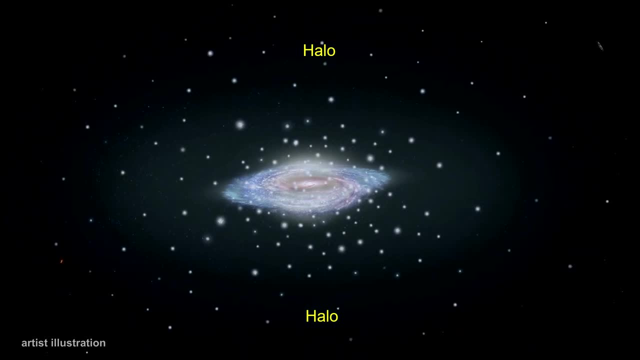 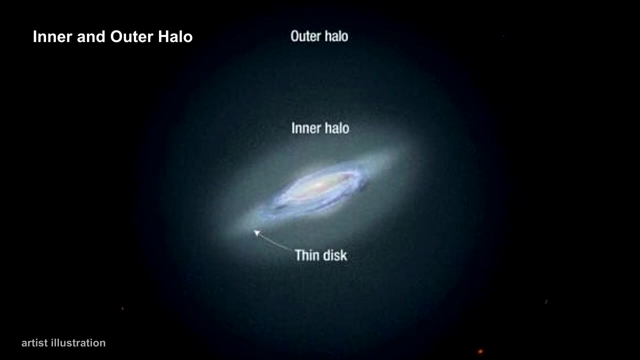 based on the locations of the globular clusters, although it may extend much further. In 2007,, using 20,000 stars observed by the Sloan Digital Sky Survey, an international team of astronomers discovered that the Milky Way halo is a mix of two distinct components. 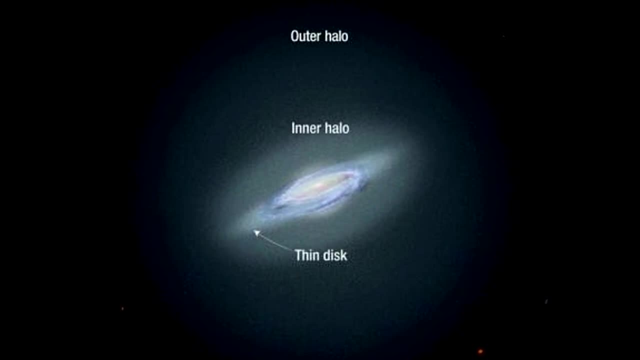 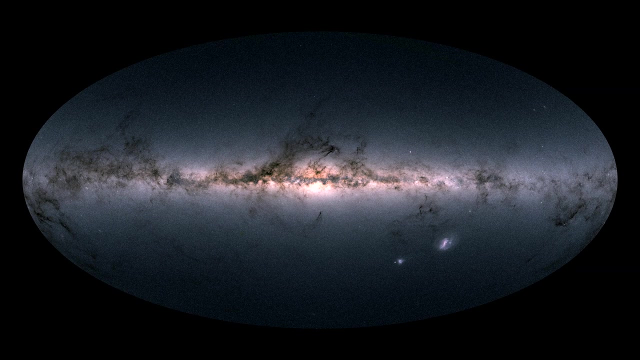 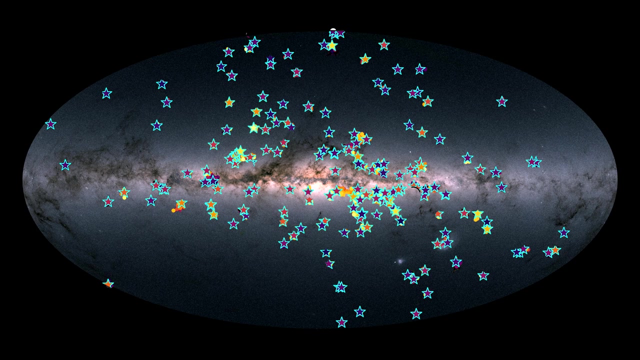 rotating in opposite directions: the outer halo and the inner halo. Then, in 2018, a team of astronomers analyzed 7 million stars from the Gaia mission and found that 30,000 of them were moving counter to the normal Milky Way flow. 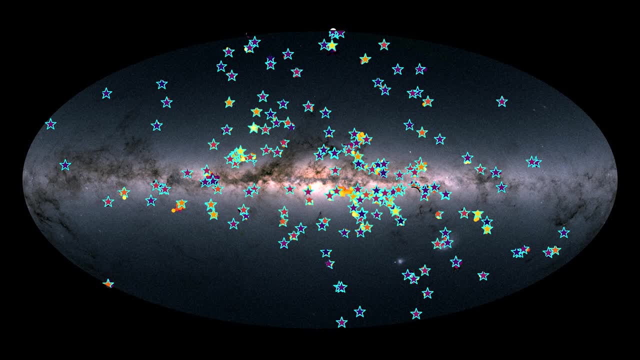 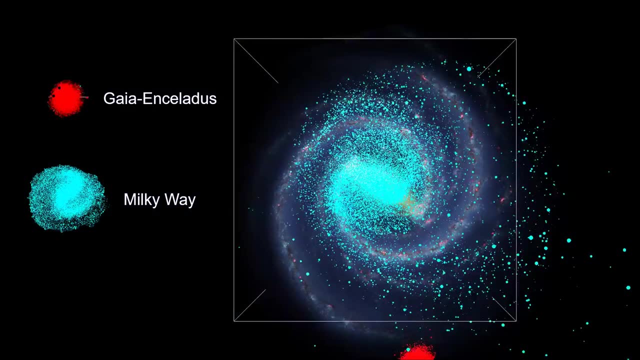 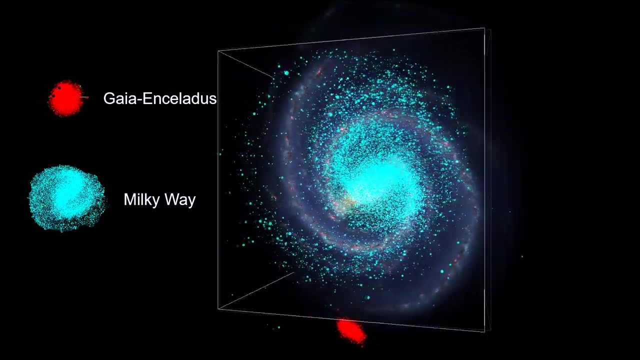 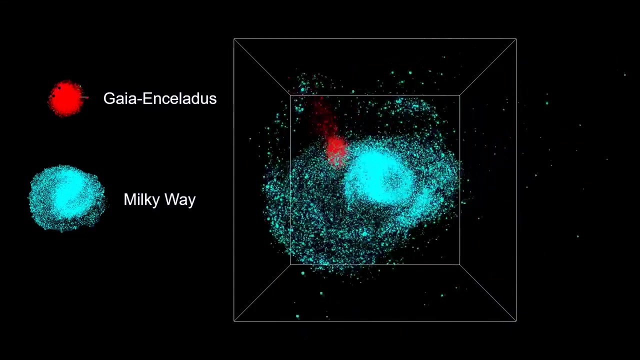 They combitated 50,000 stars to capsize them and began studies to find a universal and wide-area current within the Milky Way In 2008,. these studies indicated that these components can produce 華 and γ Star motions, and composition profiles indicated that they came from a different galaxy. 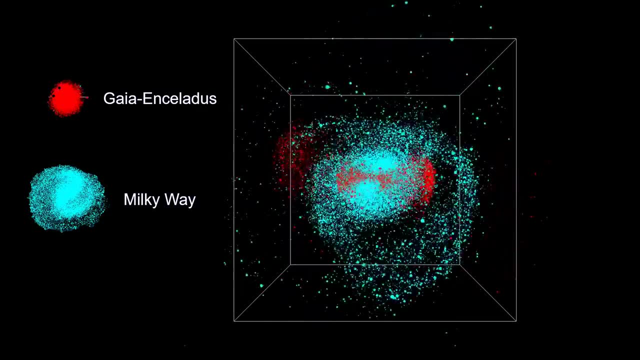 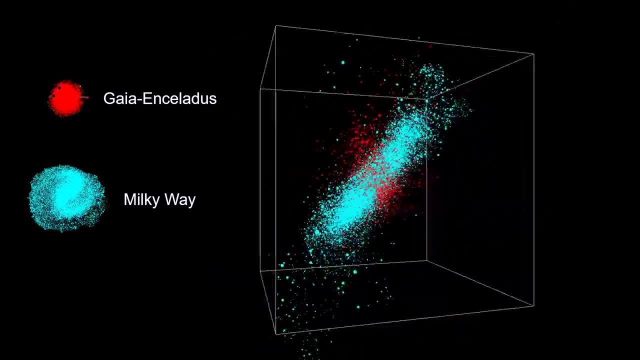 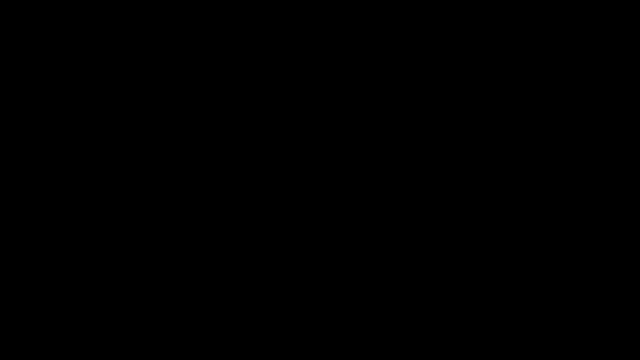 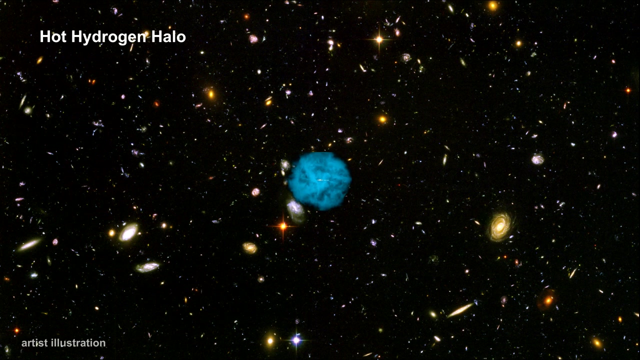 They called this new galaxy. Here we see that Gaia Enceladus is now our galaxy's inner halo. On September 24, 2012,, Chandra found evidence that the Milky Way galaxy is embedded with a large amount of hot gas in the halo. 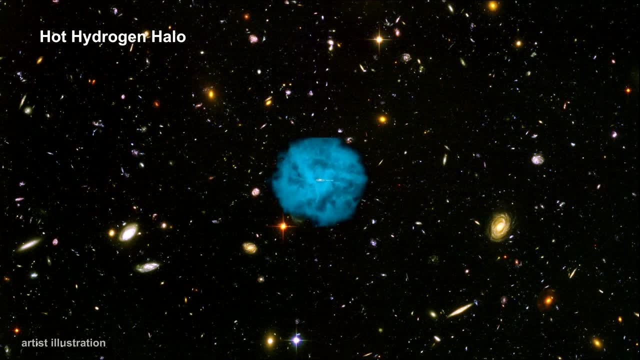 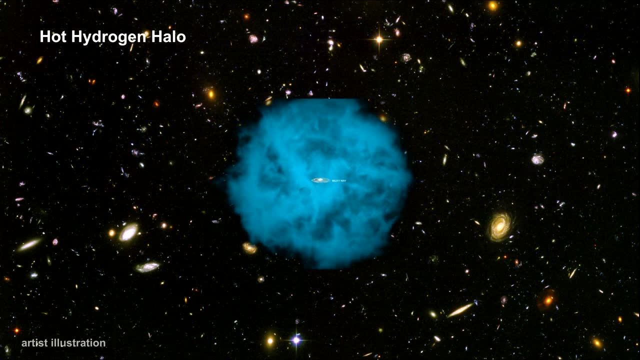 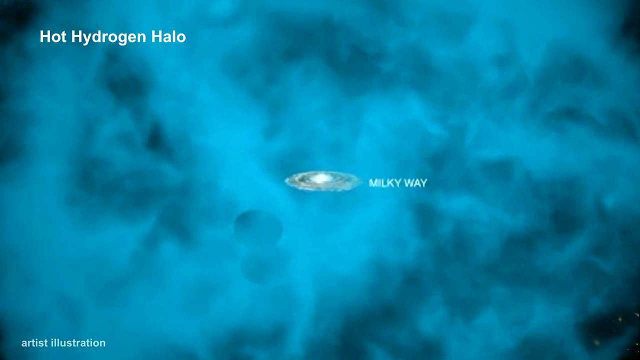 Counting this vast amount of gas. the mass of the halo is estimated to equal the mass of the stars in the galaxy. But as massive as it is, the amount of matter in this hot gas is not nearly enough to explain the galaxy's rotation curve.